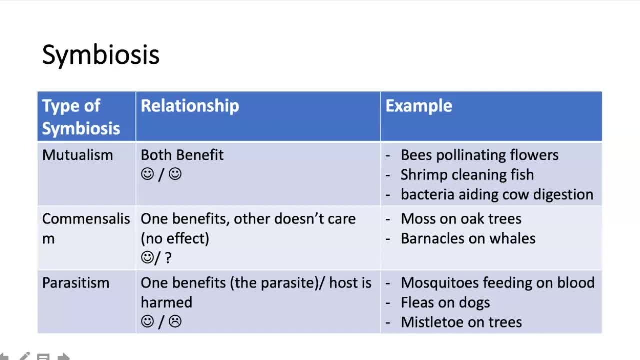 pollinating. So, for example, you could have moss hanging on oak trees. The moss is not actually taking nutrients from the oak tree, so it's not harming it. And then parasitism: you have one organism benefiting- We call that the parasite- whereas the host is the one that is being harmed. 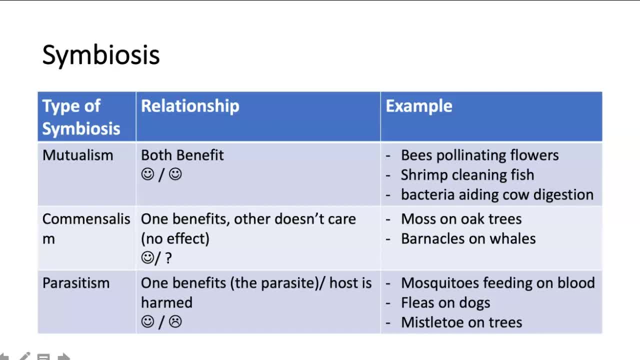 in that relationship And sometimes with parasitism, there can be more than just two organisms within that relationship. So, for example, mosquitoes feed on blood, but the malaria parasite actually uses the mosquito as a vector or transporting agent. So if you have a mosquito, 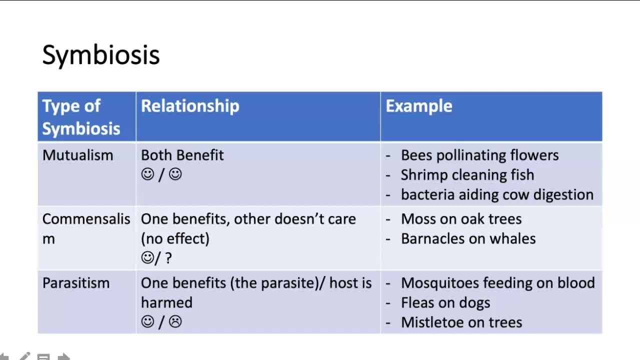 to transport itself from one organism to another organism, usually humans. in that case, Fleas on dogs is another example, as well as mistletoe on trees. Mistletoe, unlike moss, does actually take nutrients out of the tree and does harm it, So you'll often see dead areas around where mistletoe 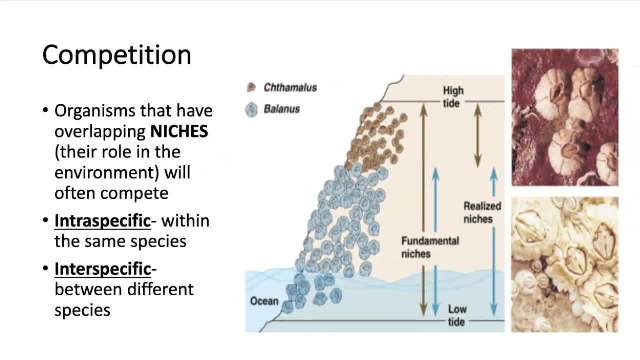 is found in trees. You're also going to need to know what competition is. Remember that overall competition is just when you have two organisms with interlapping or overlapping niches or their role in the environment that they will often end up competing. So the example that 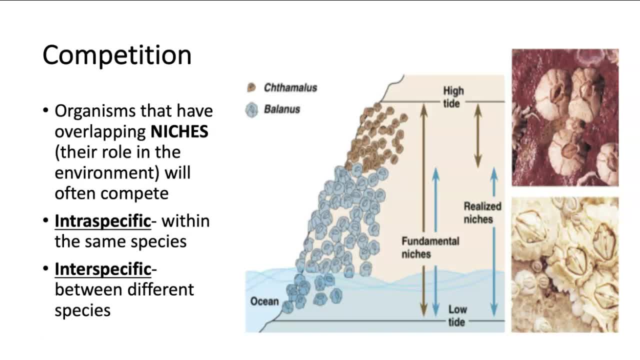 we use in class was the two different types of barnacles. We said that the fundamental niche of both of those barnacles is to cover a majority of the cliff, And so, in the case of the picture on your screen there, you can see that, with competition occurring, the blue bilanus barnacles. 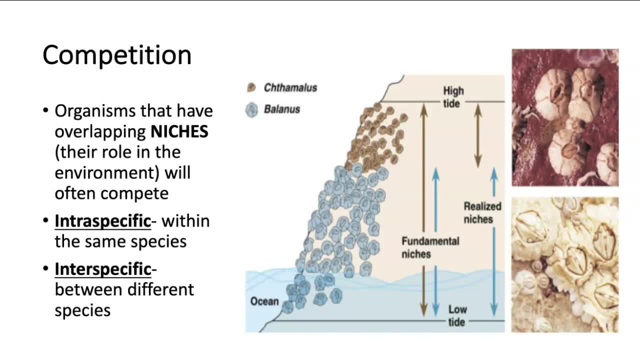 end up taking over what they prefer to have their realized niche. because they're bigger, they're stronger and it's easier for them to take over. The brown one is just the upper part of the cliff. They still will get exposed to some water. 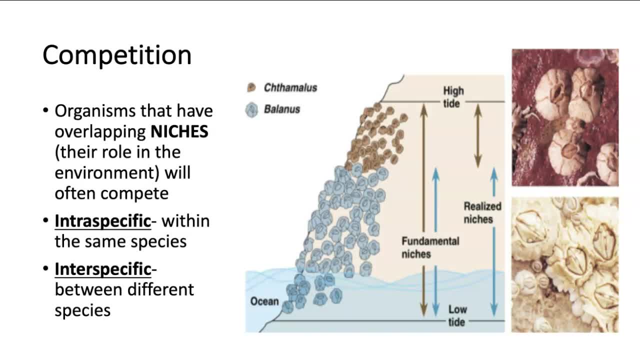 coverage with high and low tide, but their realized niches ultimately are not necessarily the same as their fundamental what they would like to have niche. You should also know that interspecific competition is when you have different species, so like with the barnacles. 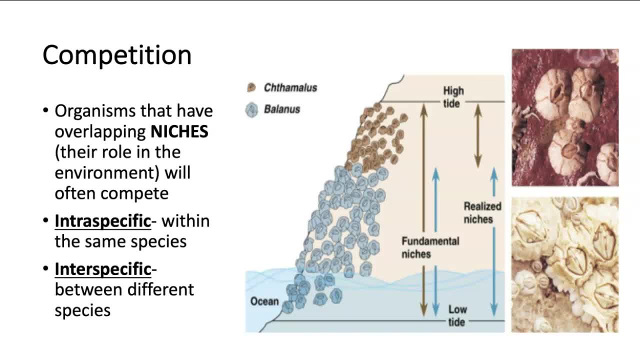 where intraspecific competition is within the same species. So, for example, two male barnacles- which is the brown one, which is the brown one, which is the brown one, wolves competing for a female wolf to mate with would be intraspecific, not interspecific. 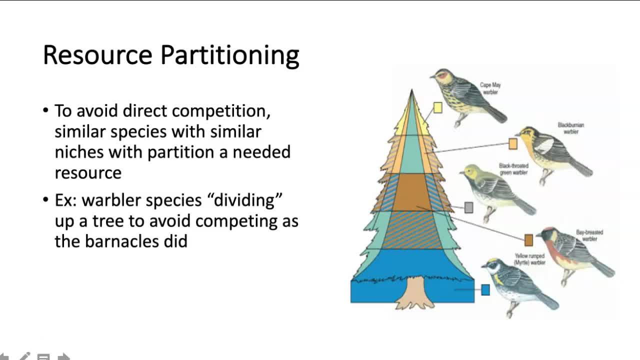 Related to your competition is resource partitioning. Sometimes, when you have very similar species, such as the warblers shown over on the right, seeking out resources within the same general location, they might divide up that location so that they are not directly competing with each other because you don't have one stronger than the other. They're all kind of. 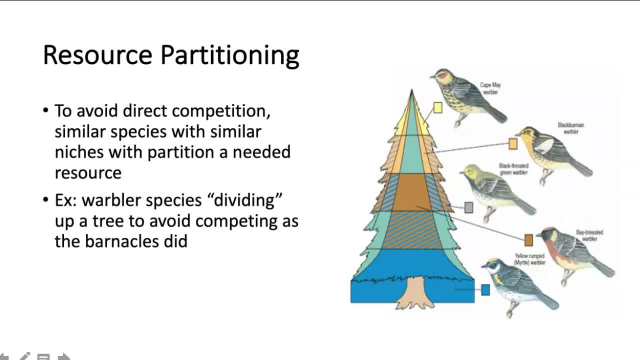 just about the same, But still need to have access to that resource So you can see where they've taken up certain parts of the tree there. like Cape May warbler prefers the upper part of the tree towards the outside, whereas the black-throated green warbler prefers the edges of the tree to the middle of. 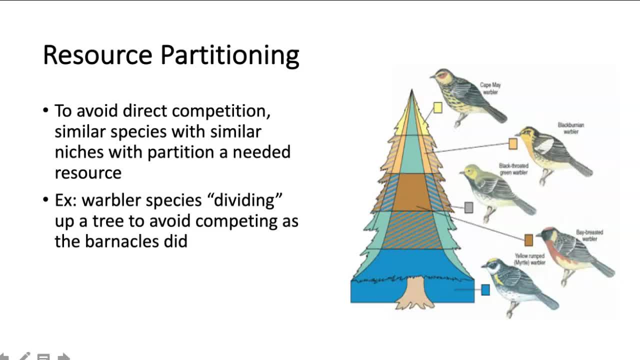 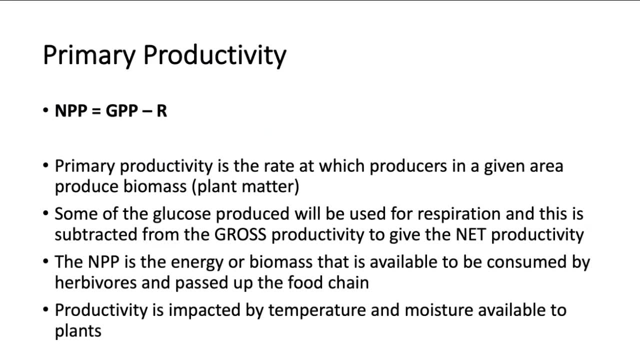 the tree. So it helps to reduce direct competition while still providing resources for very similar species. All right on to primary productivity. So you should know that GPP stands for gross primary productivity, whereas NPP stands for net primary productivity, and then R is for 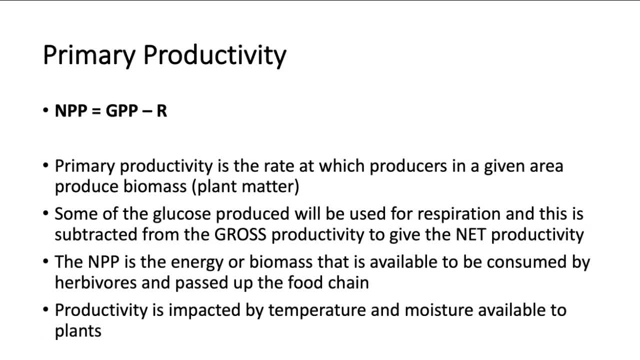 respiration. So the formula that you will need to have memorized for the exam is that NPP equals GPP minus R or net primary productivity equals your gross overall total primary productivity minus the amount of energy used for respiration by the producers that did the production of the 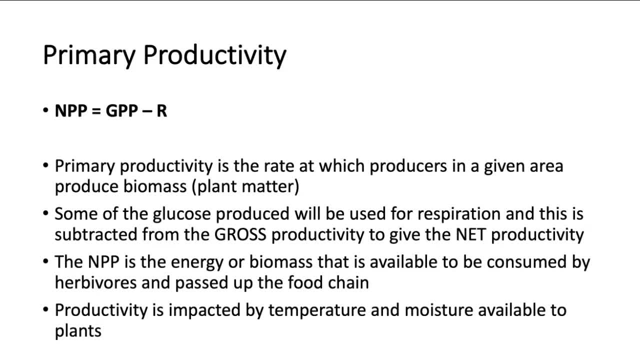 gross primary productivity. So your primary productivity in general is just how fast, or the rate at which producers in a given area are able to produce their biomass Generally. this is the plant matter, or glucose that they're making through photosynthesis. They are also going to be doing respiration, So some of that glucose. 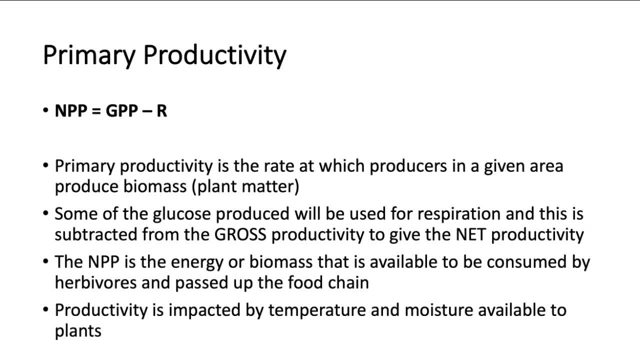 is going to be used for their own respiration purposes, to help make energy within their cells, or ATP, And what you're left with is net primary productivity, So that net productivity is the energy that's going to be available to the next level of production. So that's going to be the 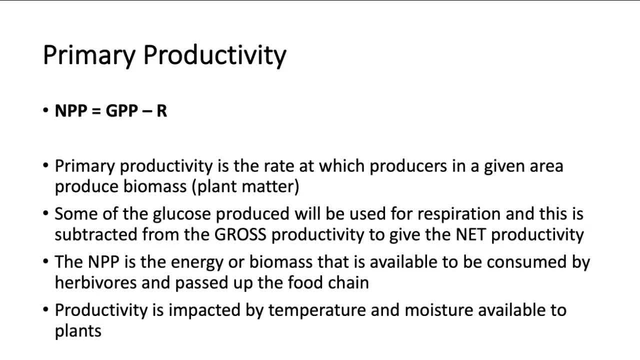 level of consumers within your food web or food chain, So usually your herbivores or your primary consumers, So that energy is going to get passed up the food chain, but you're not going to get the entire gross or overall amount of energy or biomass produced passed along. You're only going 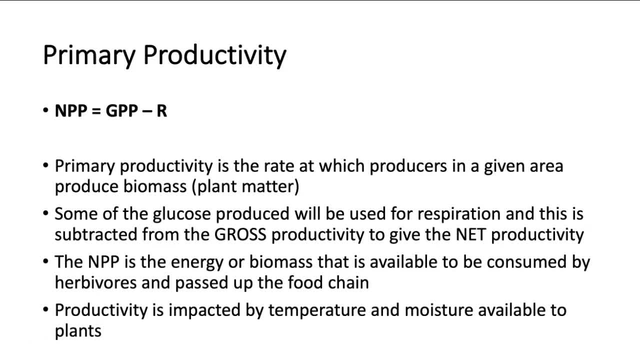 to get the net productivity passed along. And then we also talked about in class that productivity can be impacted by certain things like temperature or precipitation or moisture available to the producers within the ecosystem. So in the case of rainforests they're going to be highly productive, because it's usually pretty. 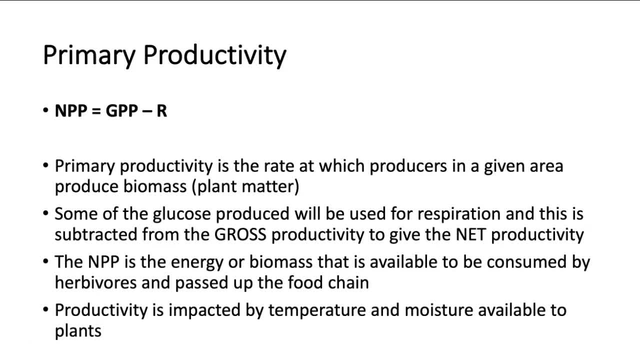 warm and pretty wet most of the time. But if you were to go somewhere like into the eastern United States, we will often see during fall and winter leaf changes where they start to change colors and the trees kind of shut down a little bit in the winter and fall because they don't have the 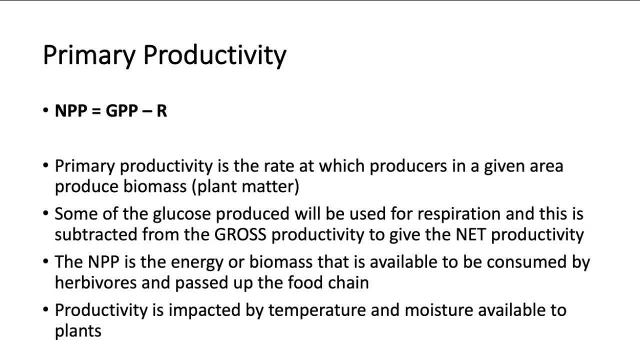 temperature and moisture availability to continue the same rate of production. So temperature and moisture are going to be key things that allow producers to produce their biomass. So that's going to be key things that allow producers, particularly plants, to produce their gross primary productivity. 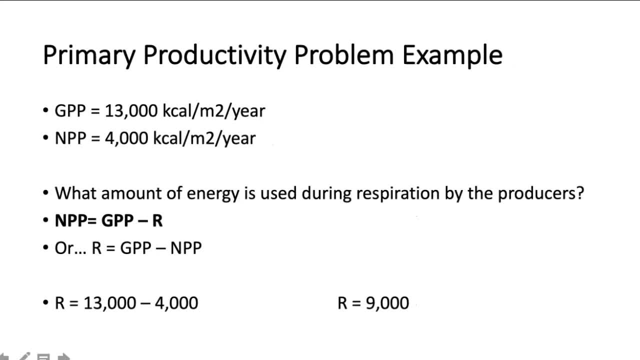 at their current rate. So part of the test you are going to have to do a primary productivity calculation. There will be one or two on there So you need to know again your formula that net primary productivity equals gross primary productivity minus respiration. But be ready to also calculate just the GPP or just the R if 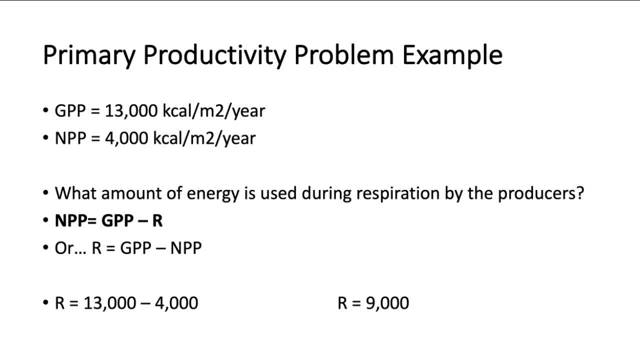 the other parts of the formula are given to you. So, for example, in this particular problem we have the gross and the net given to us and we're supposed to find the rate of respiration that is left. So you'll need to rearrange. 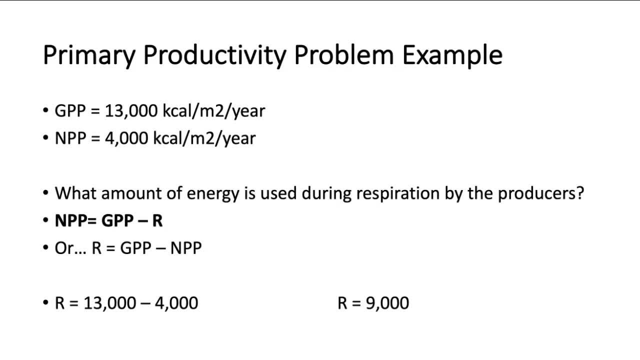 your formula. So take your NPP equals GPP minus R and flip it all around and you'll get R actually is gross primary productivity minus net primary productivity. So if we write this into our formula we would have: R equals the $13,000 of the gross productivity minus the $4,000 of the net. 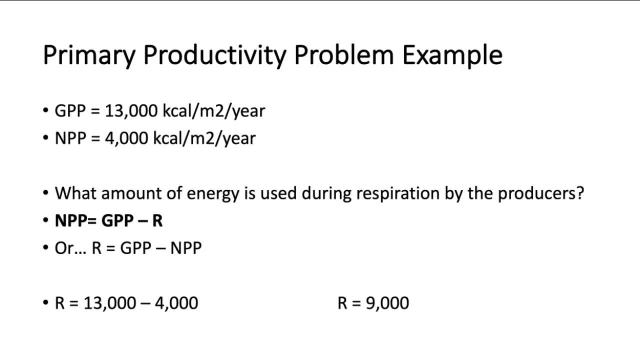 productivity. prueba net productivity, giving us a: 9,000 units of energy is used during respiration by the plants, and that is what the are. again, that formula would be. so you may have to calculate NPP, GPP or R. so make sure you know the formula and be. 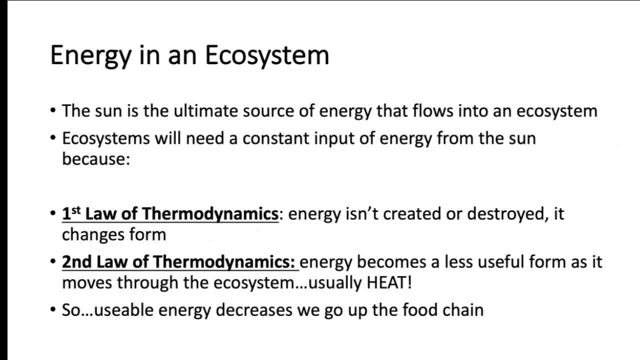 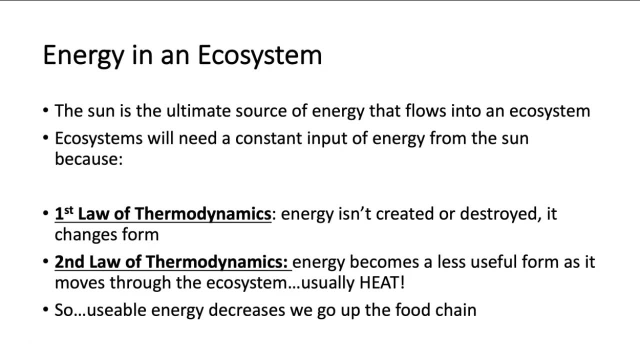 prepared to do that. all right on to how that energy actually flows through an ecosystem, you should know that the ultimate source of energy- even though we don't show it in a food web or food chain- in an ecosystem is the Sun. so the Sun is constantly in. 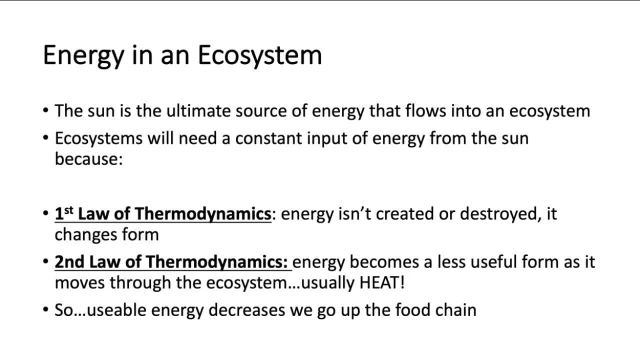 putting energy into the system, because your two laws of thermodynamics tell us that energy is not going to be a consistent thing. your first law tells us the energy is not created or destroyed. it's changing forms. so basically, we have energy flowing in from the Sun. that Sun energy is going to be used by your 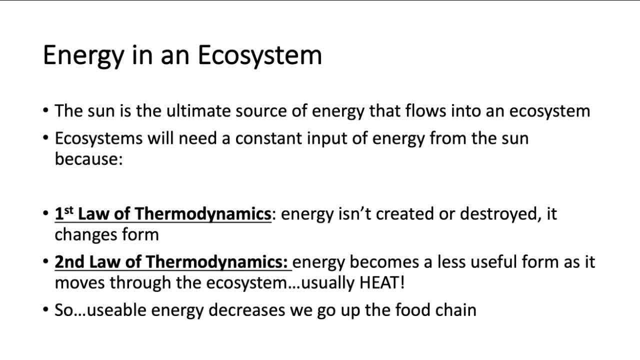 producers to make things like glucose. that gets passed along up your food web or food chain, but a lot of it is lost, usually to the form of your ecosystem heat or waste. That's your second law of thermodynamics, So energy tends to become less useful as you move through the ecosystem, from producers up to your top level carnivores. 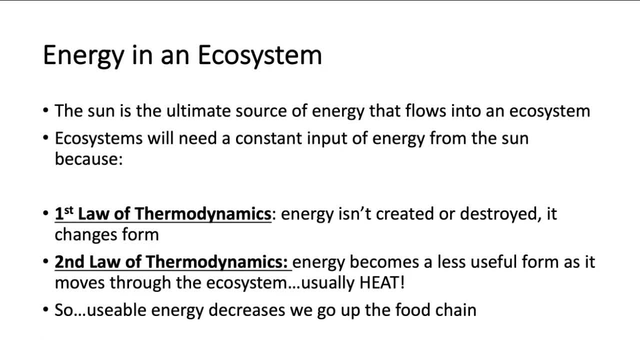 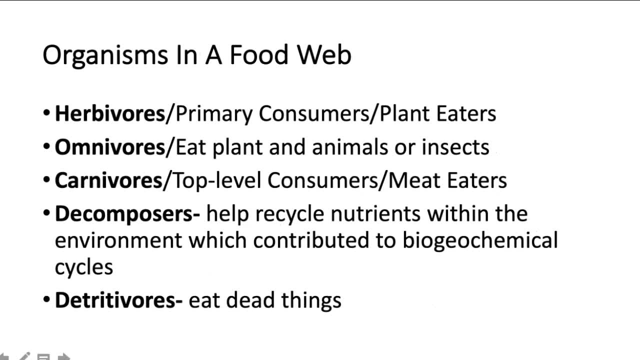 and that useful energy is going to be decreasing Again. we usually lose about 90 percent of it to heat. Here's a quick review of a few of the organisms you're going to see in a food web before we apply some of that energy knowledge. we just got to an actual food web and energy pyramid. 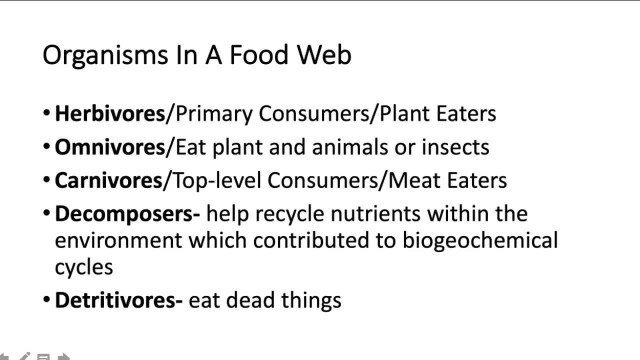 So herbivores- remember. herbs are plants, so herbivores are plant eaters. They're usually also your primary consumers- Omnivores- omni means everything, so they are going to be your everything eaters. Your plant and your animal are insect eaters. Remember, insects do technically 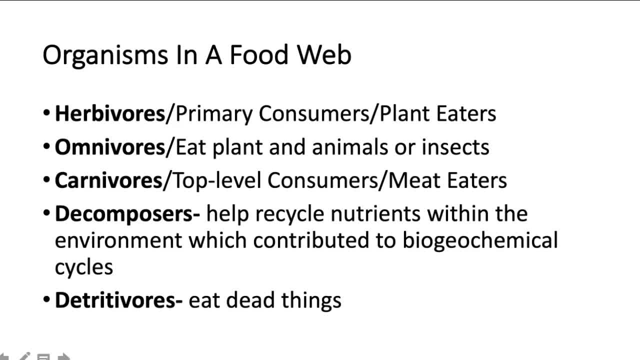 qualify as meat, And then carnivores. remember carny, so carne in Spanish means meat. Hopefully you learned that from your Spanish class. So carnivores are going to be your meat eaters or your top level consumers. Usually, they're going to be either a 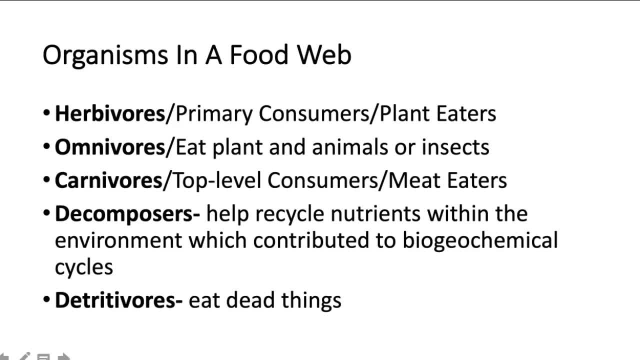 secondary, tertiary or quaternary level consumer, So higher up in your food chain or food web. Then we also have our decomposers and we have our detritivores. So decomposers usually break down dead things. things like bacteria, mushrooms or fungi would be doing this. 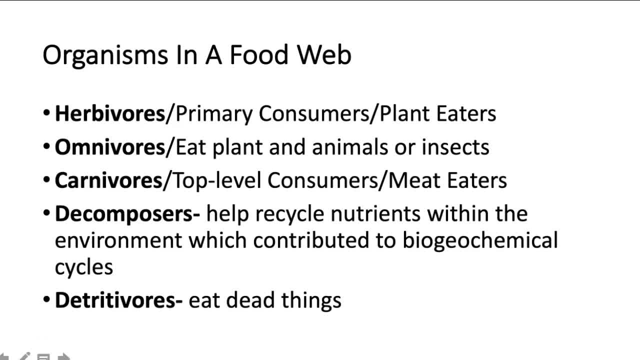 And they are going to help recycle nutrients through the environment, So they're usually contributing quite a bit to your biogeochemical cycles. So think of like nitrogen, for example, being decomposed from an old dead plant that's being broken down by maybe a mushroom in a 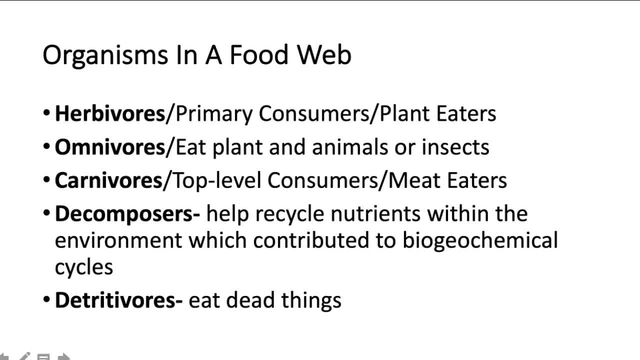 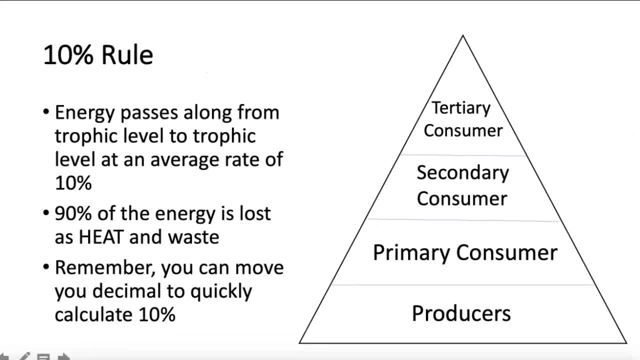 forest. And then detritivores: they eat dead things. The term detritus literally means dead stuff in an ecosystem, So detritivores are eating your dead stuff. Okay, So for the 10% rule, remember that this is an average rate of the amount of energy passed among your trophic levels. 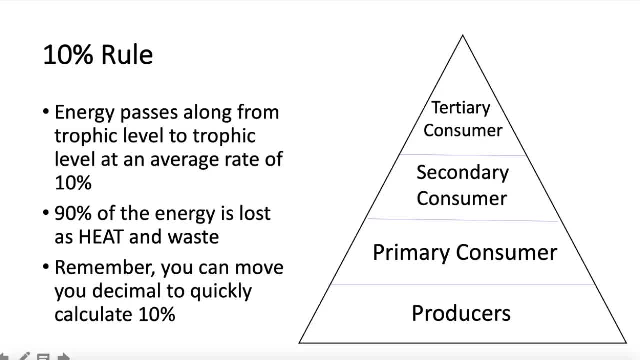 on your food chain or, in this case, our energy pyramid. So on average, as we go from one level to the next, we are going to have about 10% of our energy Passed along. It's not always that much. We did some problems in class where sometimes it can vary. 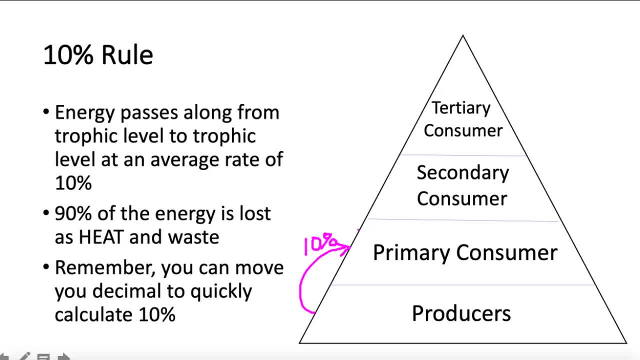 a little bit, but it is 10% on average. Then, from primary consumer to secondary consumer, we would have, for example, whatever is available at primary passed along to secondary at a 10% rate, and then secondary to tertiary. about 10% of your energy is going to be passed along. 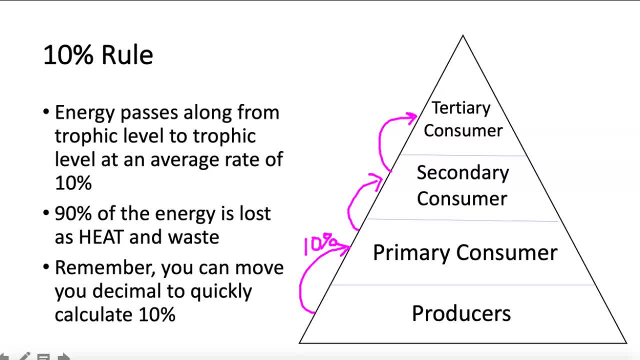 as well. So as you are going up your food web or food chain, you can see we're going to have a decrease in energy, Hence why we use this pyramid or triangle shape. So about 90% of your energy is going to be lost, So we're going to have at each 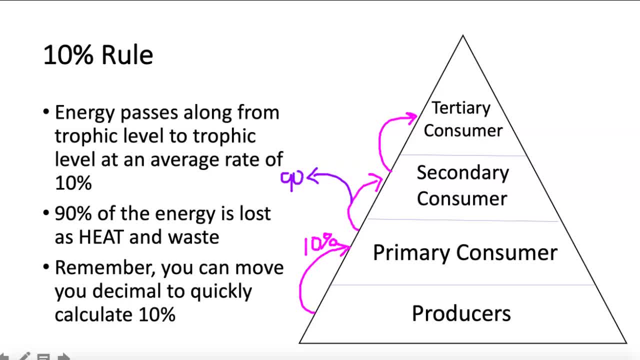 level 90%, leaving usually in the form of heat. So 10% gets passed along, 10% gets passed along, 90% is lost to heat and to waste. You should be able to do your 10% calculations, So remember. 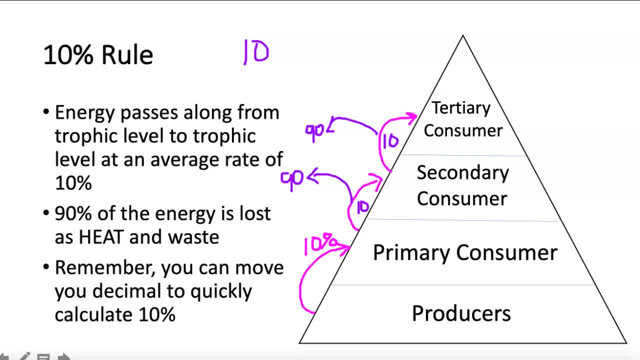 the easy way to do that is, if you have, for example, 100 units of energy, let's say at your producer level, and we want to know how much is at the primary consumer level, you move your decimal in one. and if we had 100 again at producer? 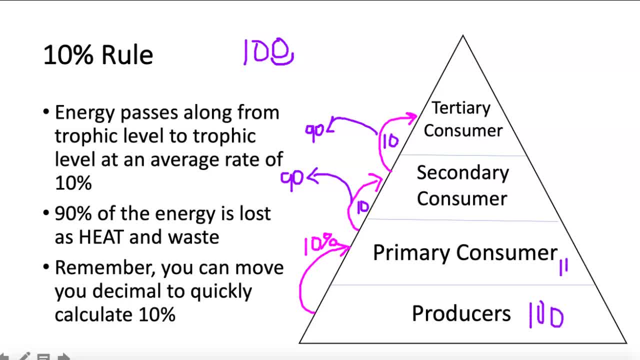 we are now going to have 10 at the primary consumer level. The other 90 is lost to usually heat If we move it in one more than at our secondary level. we would just have one If we were to move it in one more at our tertiary level. 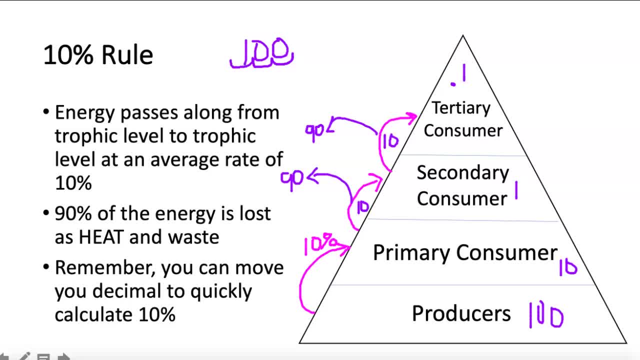 have 0.1.. So make sure you're able to do those 10% calculations. And then you will also need to be able to tell me how much energy is lost. So if I ask how much energy is lost between the producer to the secondary consumers, you would take 100 and you would subtract. 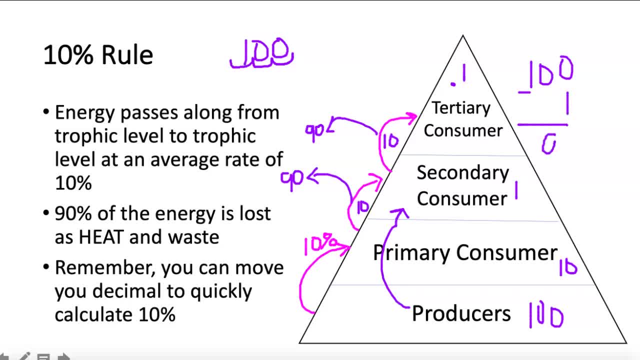 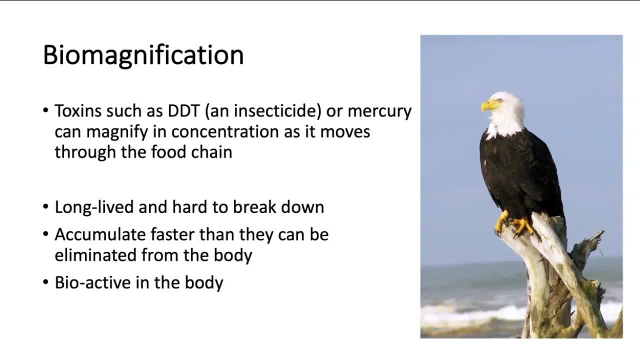 one, And then the amount of energy lost in those two jumps up the food chain would be 99.. All right, last thing we need to make sure we know for the exam is biomagnification, which we talked about in class in reference to DDT. DDT is an insecticide. Mercury is another compound that is.